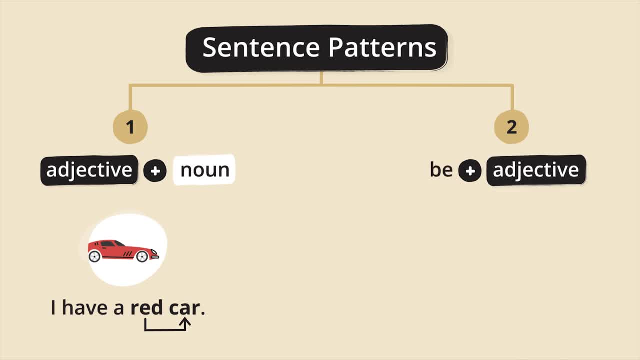 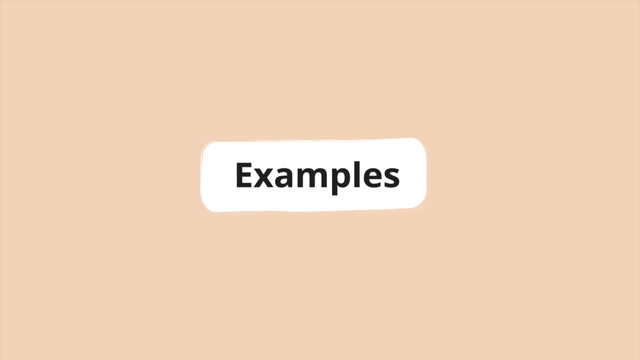 In this pattern the adjective follows the be verb and describes the subject noun in the sentence. For example, in the sentence the student is tired, The adjective tired follows the verb is Tired, describes student. Let's look at some more examples of adjectives in a sentence. 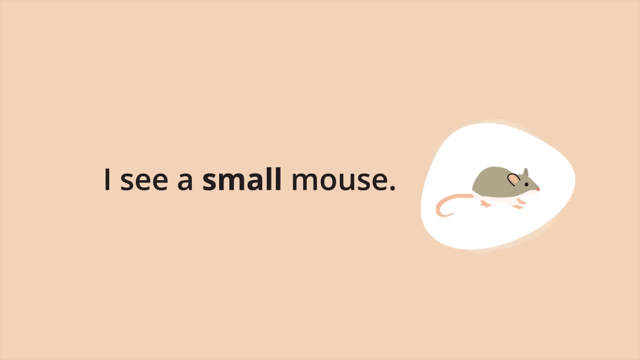 I see a small mouse. That is an expensive car. The children are happy. The pasta is delicious. They live in a big blue house. My new boots are tall and high. I see a small mouse. That is an expensive car. The children are happy. 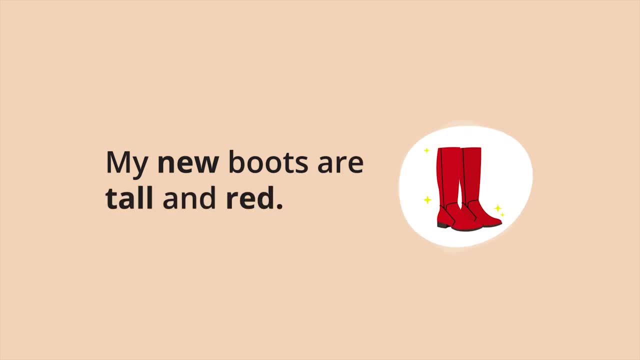 The pasta is delicious. My new boots are tall and red. Did that? Now look at the picture and unscramble the words to make a sentence. Say or write the sentence. For example: the apple is red. Now you try. 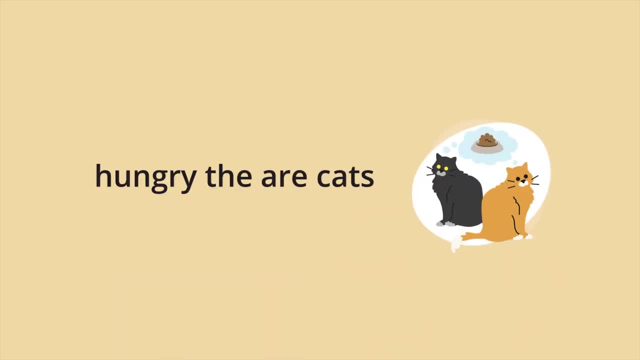 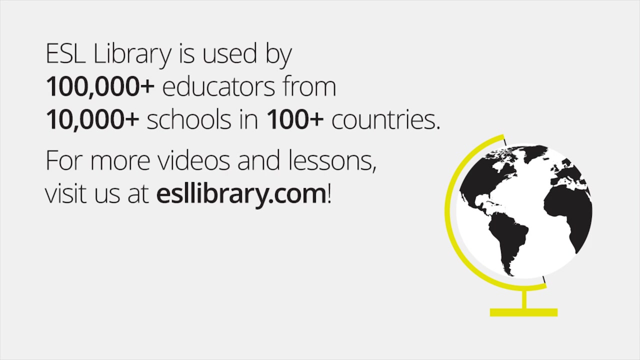 Meow, Meow, Meow, Meow, Meow The end. Thank you for watching. Thanks for watching. Thanks for watching.